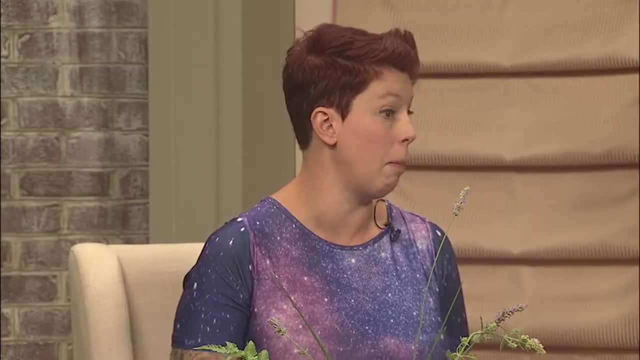 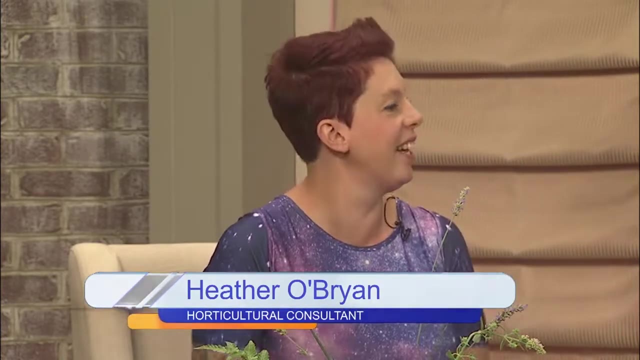 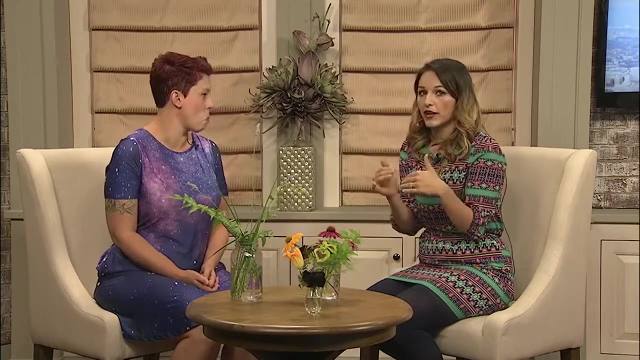 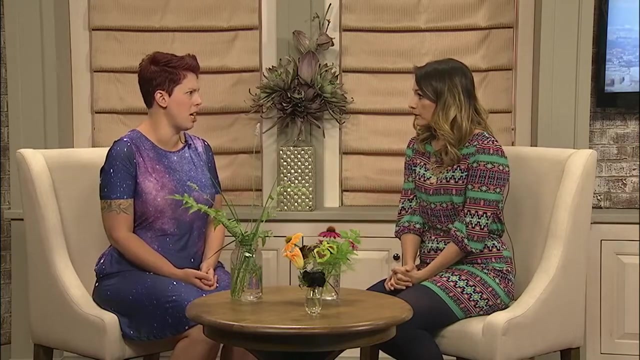 Plants serve many purposes in our lives, like air production, pollination with bees and that sort, and without those two things we would not be here, Absolutely. You know, that makes it kind of important. You actually have a fun way to kind of introduce this to children and it's, I mean, just looking at it, it sounds perfect. I have a five year old and he would be so into this, and you go kind of by the senses. Yeah, the five senses, although sound is kind of hard. We'll touch that later. Yes, Okay, so let's. 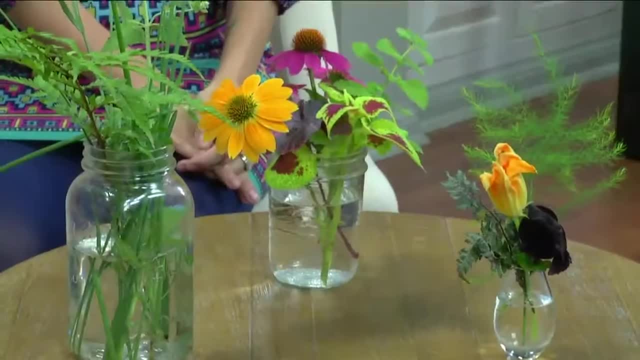 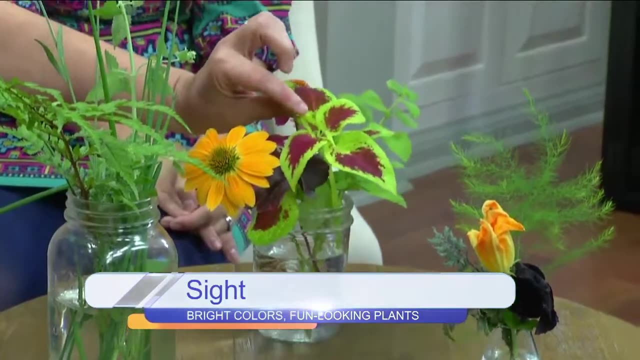 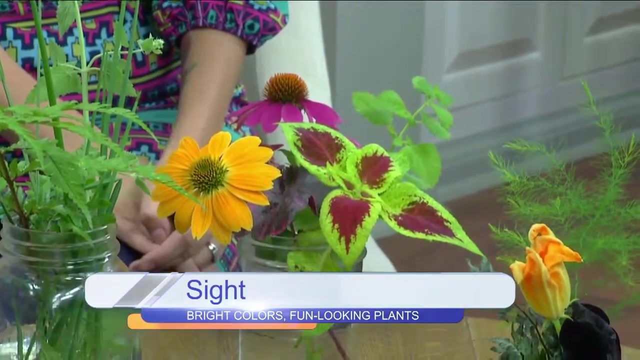 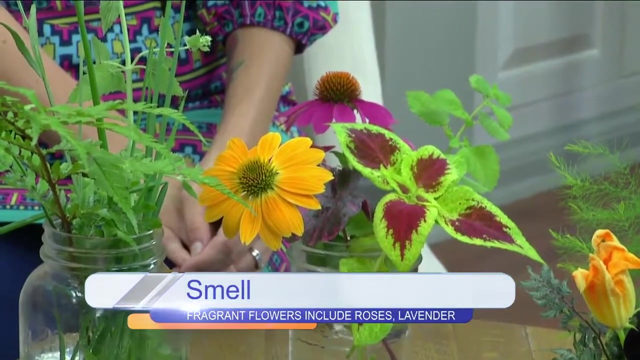 jump into it. So sight: obviously, if we have children that have sight, it's the easiest because there are colors galore. I've got coleus here, which is really bright colors, and echinacea here as well. If your children aren't sighted, the other senses are going to come into play even more, Right, Yeah? So our next one is: let's see smell. Yes, So herbs are always a good thing for smell, Right? This is 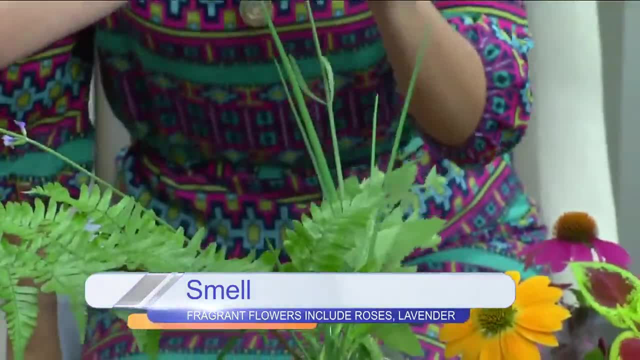 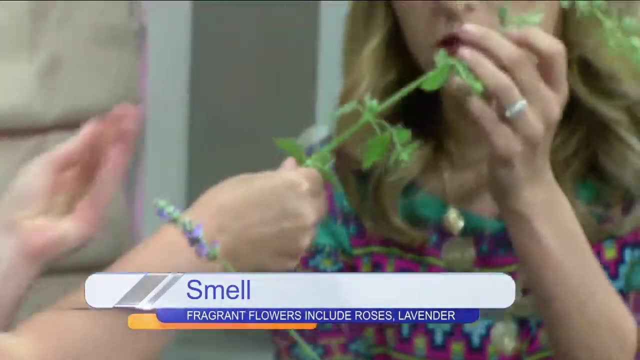 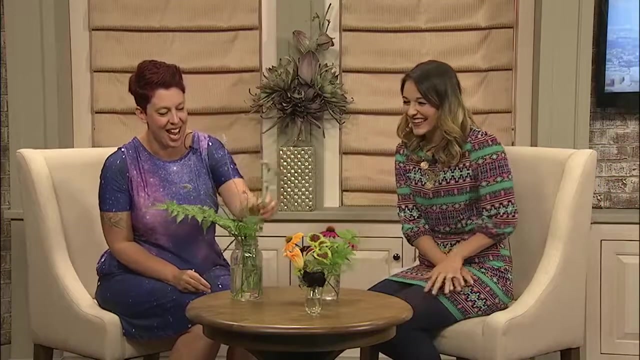 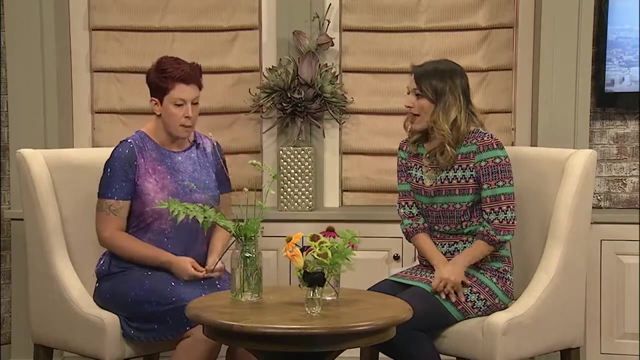 tell me what it is. Smell it: Lavender, Lavender. Oh my gosh, that smells amazing. So you want to do good smells and then you want to do funky smells. Uh, oh, funky smells. Smell that one. Oh Oh, This is cat mint. I know I fooled you. This is cat mint and the cats go nuts for it. It's also really good mosquito repellents. Oh, I like that. They don't like funky smells, Right, Okay, Alright, so that's smell. and then this is what I was. 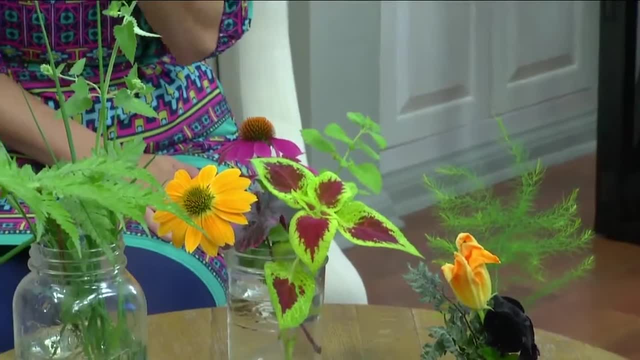 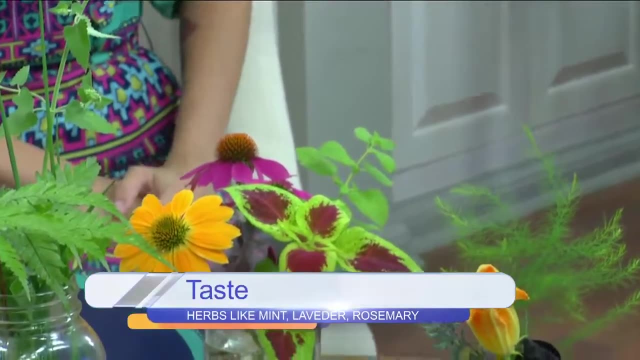 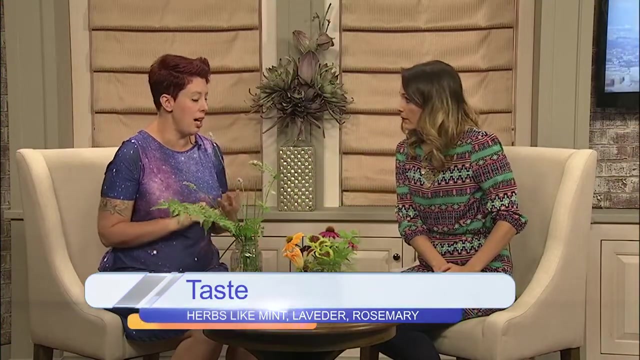 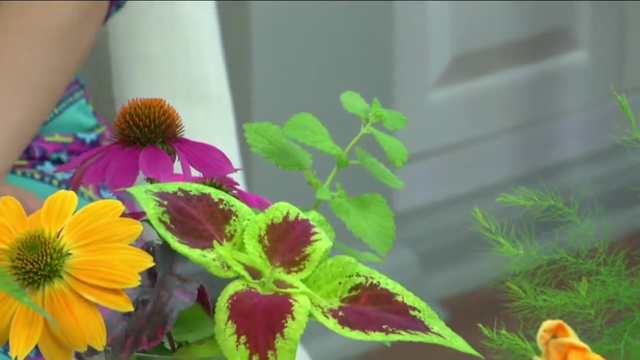 smelling earlier. right, What is this one? That's lemon balm. Lemon balm smells like lemon and it tastes like lemon, Which leads us to taste: Okay, I can eat this. Yeah, I will. It's good in your salads, Oh It's. Wow. Yeah, That is crazy. Very lemony. You can infuse it in water. You can infuse it, and you can use it instead of lemon in your teas and all kinds of stuff you can do with lemon balm. That's great. Okay, I've got chives here too. you can taste, but it just tastes like onions. Okay, and then we